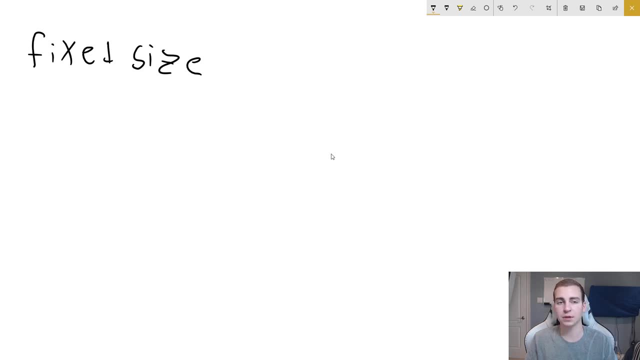 and you don't know how big it's going to be, how do you decide? Well, that's typically when you might use a different structure. But anyways, that's something to note, that you have to pick how big it's going to be before you even, you know, create the array. Now the next thing with 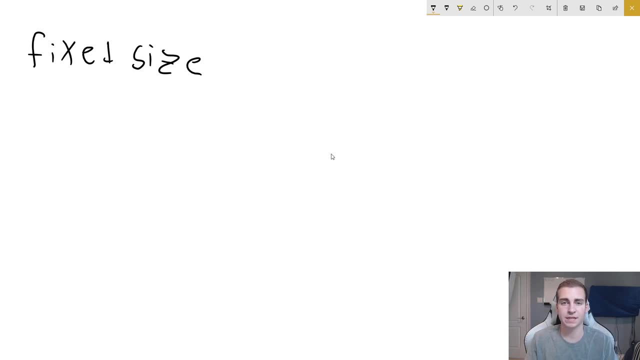 this fixed size is that, if you'd you know, say, you create an array- that's something you know- size 10. And you now want to add an 11th item to it. Well, you can't do that, because there's 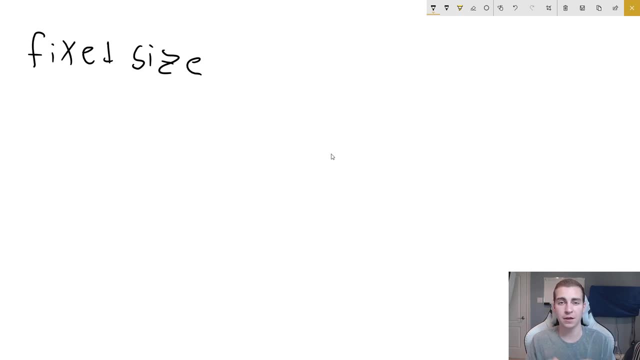 no more room in the array so it can be filled up. And another thing with this fixed size is that, say, you create an array and maybe you're like you know what: I don't know how big I want this array to be, but I'm going to make it size 10,000. So that's just massive. 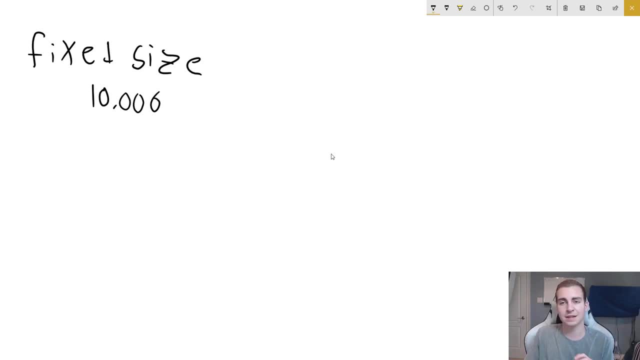 enough that I don't have to worry about it. Well, if you do that, that's another really big disadvantage, because what you've actually essentially done here is you've put a little slot of memory here- and I'm just drawing like mock computer memory- And you've said: 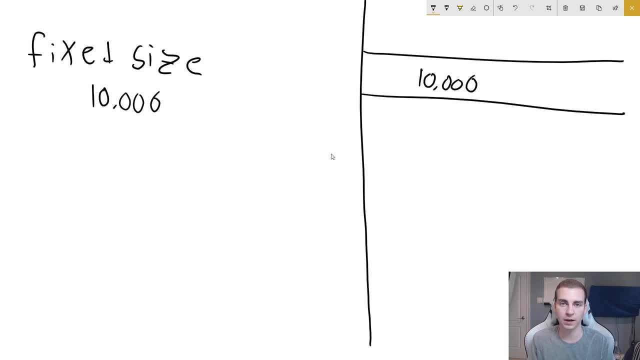 I'm going to make sure that I have 10,000 spaces for items in my computer memory, which means that you're actually locking up a ton of memory- And this is known as a memory leak- by creating such a massive array that you're not actually going to use. So when you only 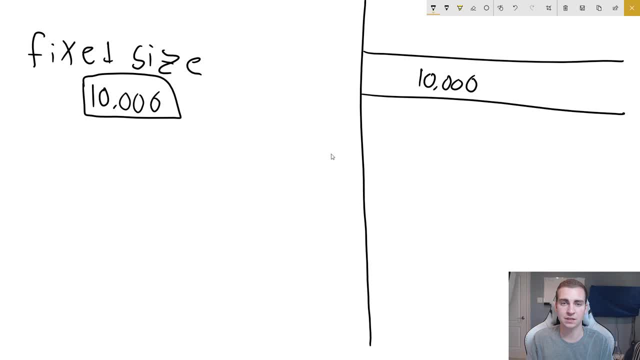 have a few items in a really large array. that again is another disadvantage of an array, because now you're using all of this space and memory that could have been used for something else. Now, in modern day computing, with people having 16,000, you're going to have a lot of space in your memory and you're going to have a 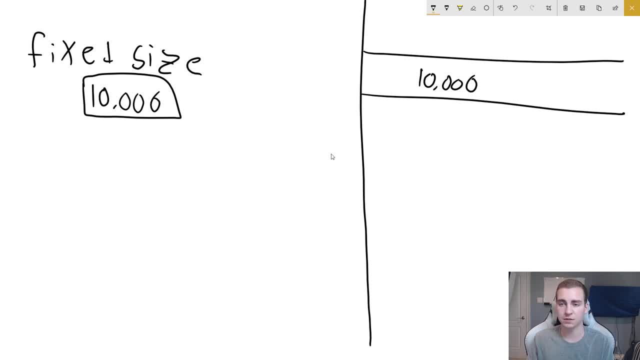 32 gigabytes of RAM in their machine. it's not really a huge issue, but still something to think about when using an array. Alright, so now we talked about a few disadvantages of it. What's one of the advantages of an array? Well, one of the advantages is the 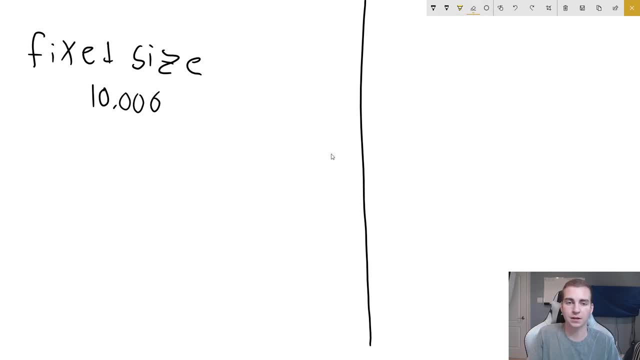 fact that you can index items. Now, a lot of people take this for granted, But we know that we're using an array, we can use something called indexes And we can look up any item in our array by simply knowing where it is And that position is being held in our computer. 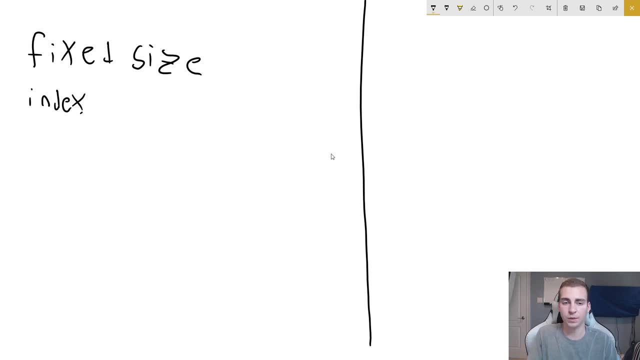 memory because of this fixed size. Now, when we look up an item, this actually happens in what's known as constant time, which is very fast, as fast as you can do something in computing. So, because we have this fixed size in our memory, let's say we have an array of size five, so 123455 squares. 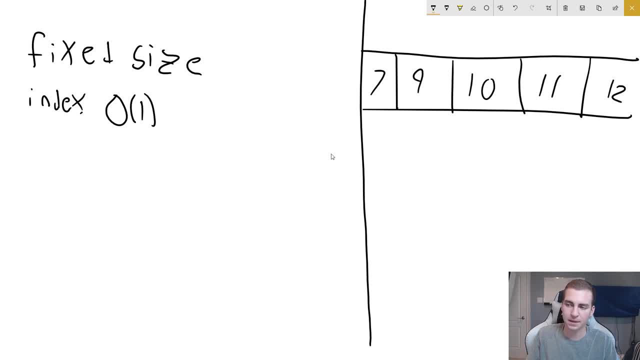 and maybe these are items here like that. Now we know that the indexes go from zero all the way up, And if I want to look up any item, all I have to know is where it is. So like index three, and I can grab that immediately, as opposed to using something like a list that takes. 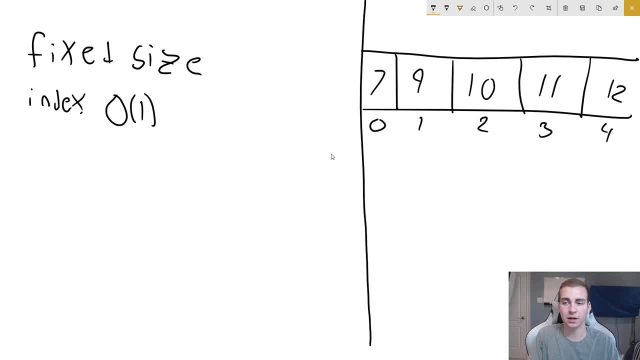 a lot longer to do that. So that's something to remember: that indexing items and getting any random item takes, Oh, one constant time. Now, what about inserting, deleting and removing items? Well, let's look at how that works, because it's not quite as fast Now, because 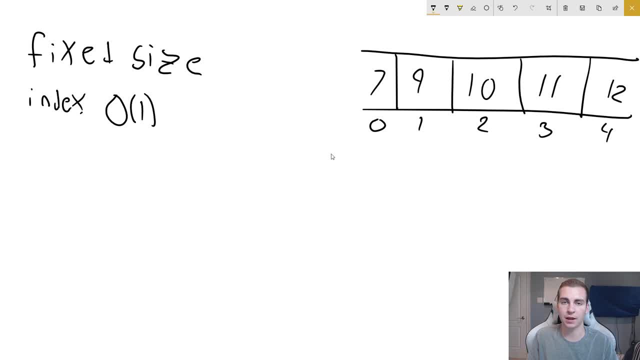 of this fixed size in our memory. if we want to insert an item, this is actually quite computationally heavy. Let's say, we have this array and we want to insert- I don't know- item five in between seven and nine. Well, to do this we actually need to shift every. 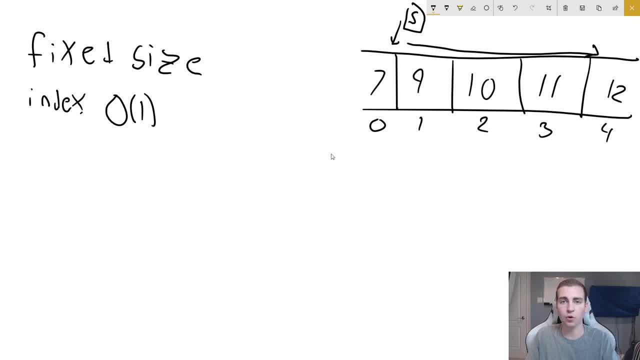 single item in our array past this point over And we might even have to remove the last element to make room for this new inserted array. So when we do that, it looks something like this: we have the box seven, which is index zero. we now squish in our new index. 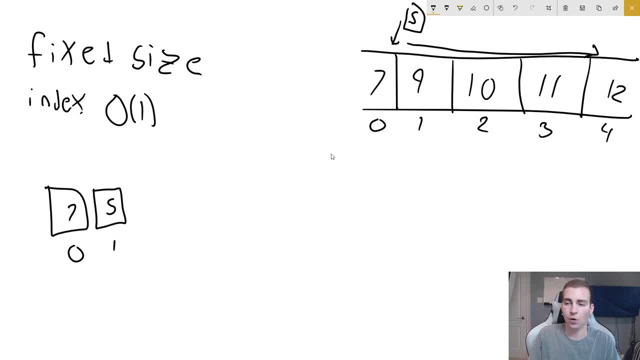 five, sorry, new item five, which is index one, And now all of these indexes need to be incremented by one and shifted over. So nine needs to go where 10 is, 10 needs to go where 11 is, and 11 needs to go where 12 is, and 12 is well lost in emptiness. it's gone forever, Right? 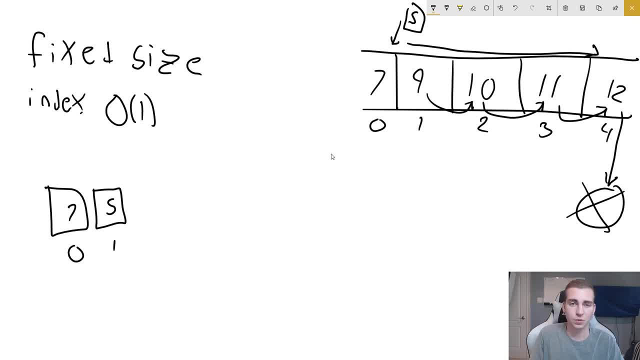 And that's what happens when we insert an item, at least into a full array. So that takes what's known as Oh and time, which is a long amount of time in computing, based on how big the list is or how big the array is. it's going to continually take longer. 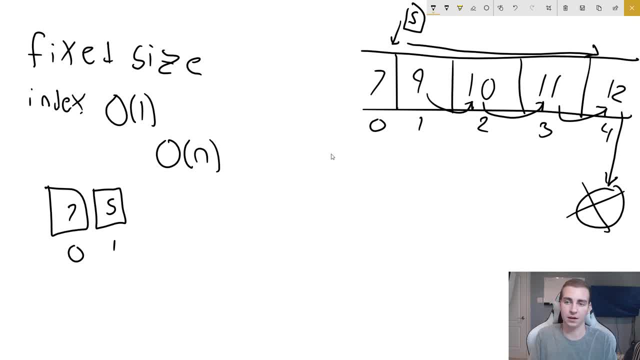 and longer to insert an item, especially if that item is at the beginning of our list. So once we insert that item, that was a horrible box. I'll redraw that one. we have nine, we have 10. And we have 11. But these are now moved to new indexes. So two, three and four.